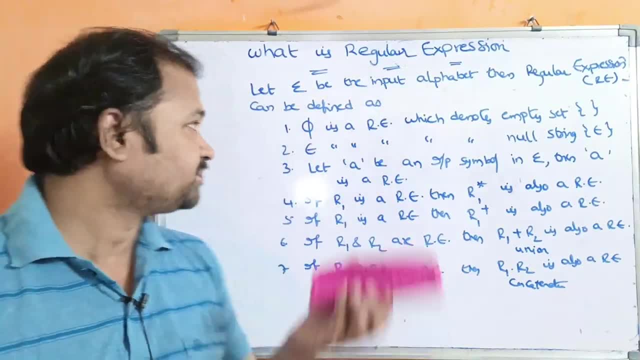 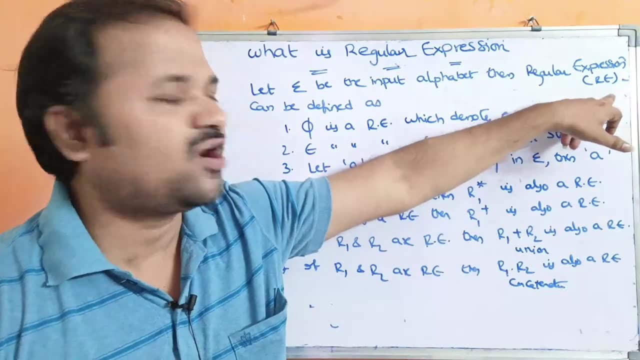 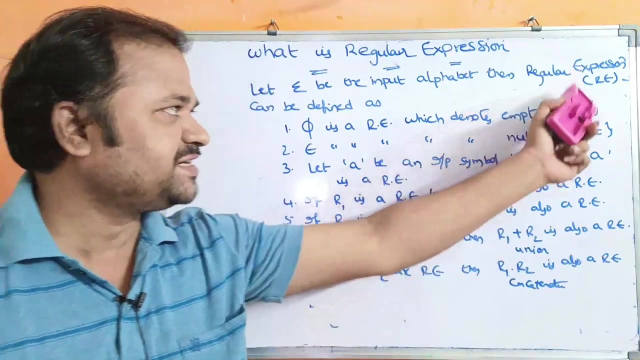 Now let us see the definition for the regular expression. Let sigma be the input alphabet, Then the regular expression. In short, we are calling it as RE for space constraints. In the examination you can write regular expression also Here for space constraints in place of. 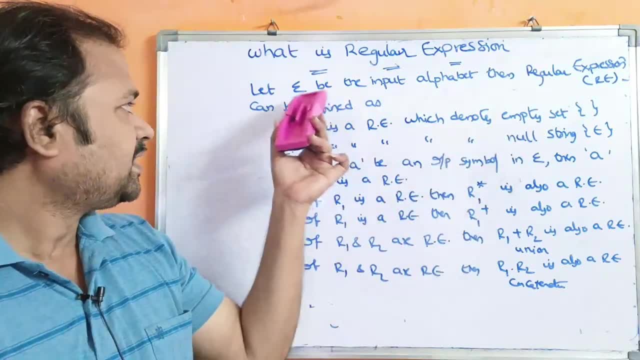 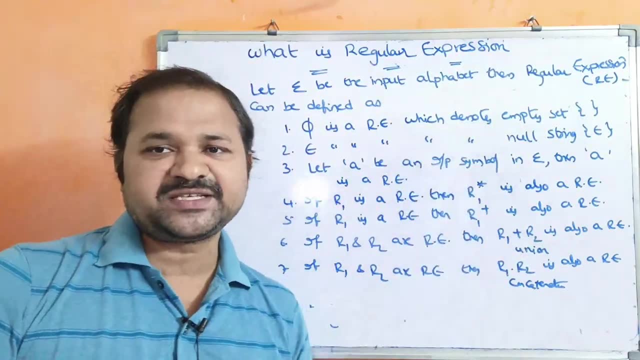 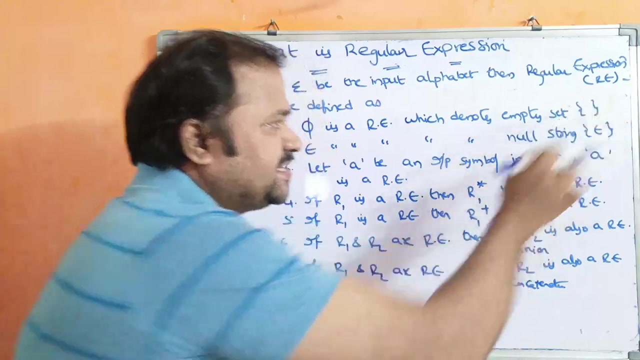 regular expression. I am writing RE. If let sigma be an input alphabet, then the regular expression can be defined as: Totally we have seven points at it. The first point is: pi is a regular expression which denotes empty set. So pi means empty set. 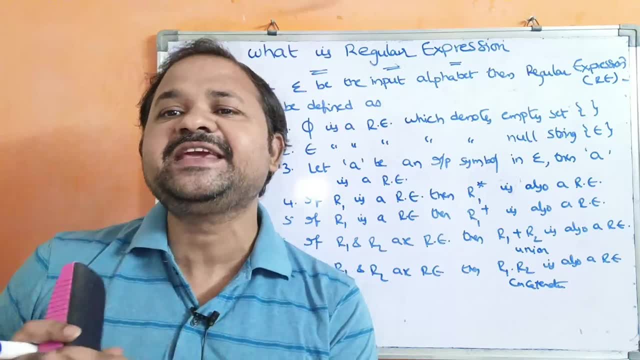 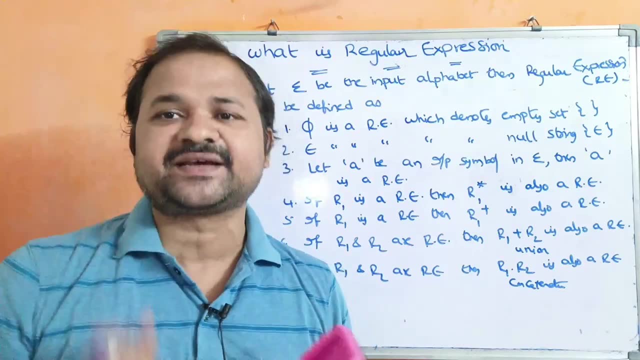 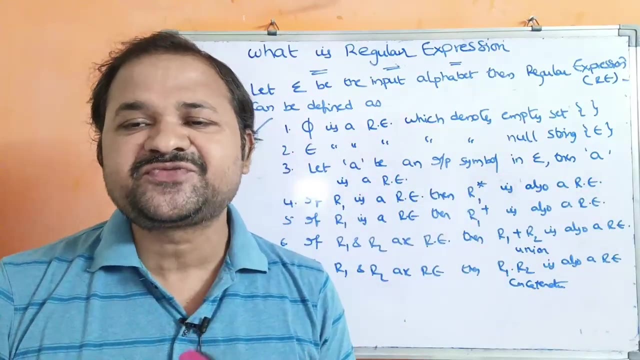 Empty set means the set does not contain any elements. So if we have empty set, then we can represent that empty set by using regular expression as pi. So pi is nothing but a regular expression which is useful in order to represent empty set. Empty set means: 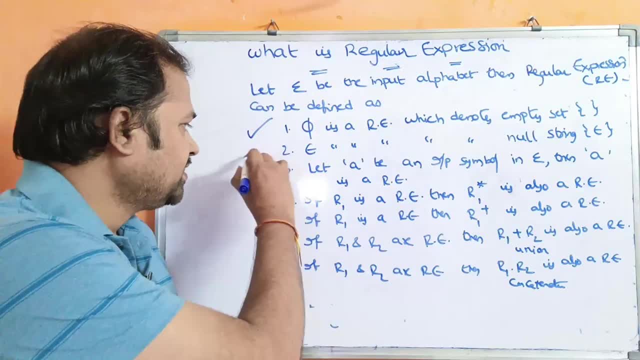 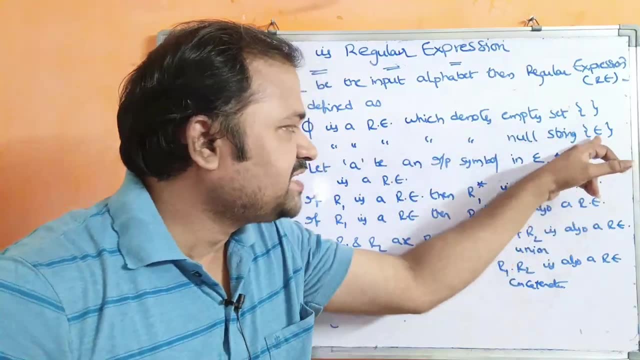 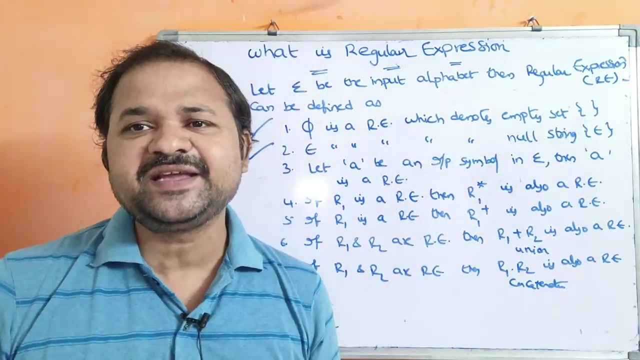 the corresponding set doesn't contains any elements. Next, second rule: epsilon is a regular expression which denotes null string. Null string means within the curly braces, epsilon. So null string is represented like this: So null string means we have a string, but length of the 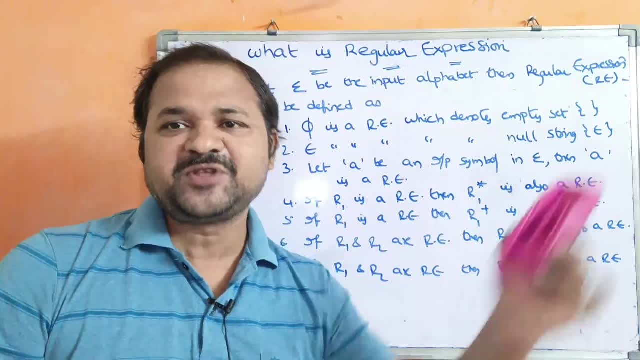 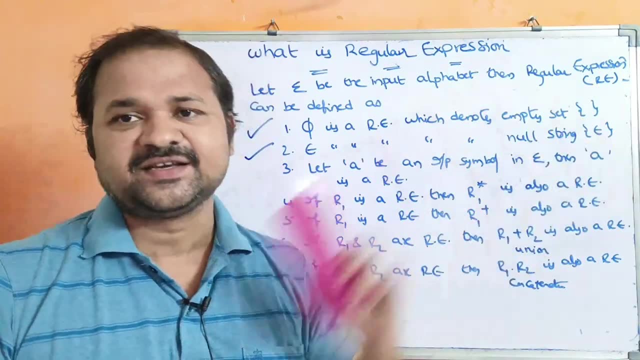 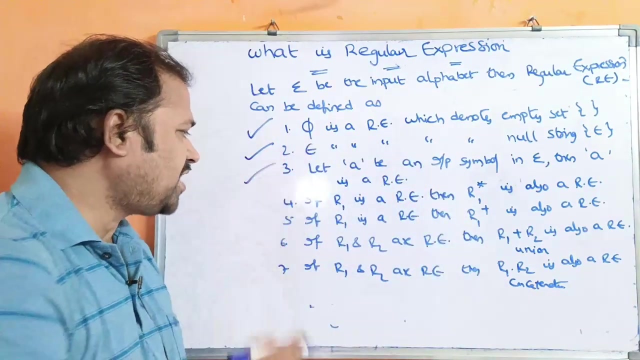 string is 0.. Here we have epsilon. Epsilon is the string, but what is the length of that string? 0 is the length of the string. So if we have a null string like this, then we can represent the regular expression by using what Epsilon. Now let us see the third rule. Let a be an input. 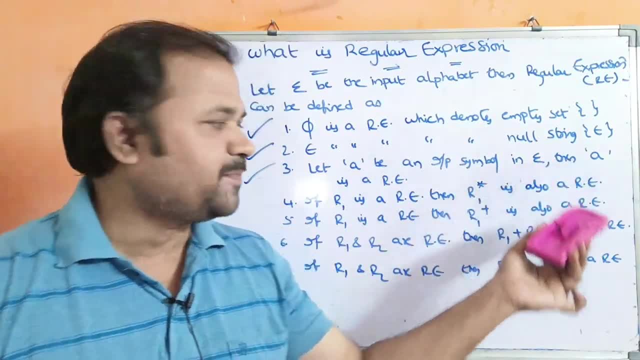 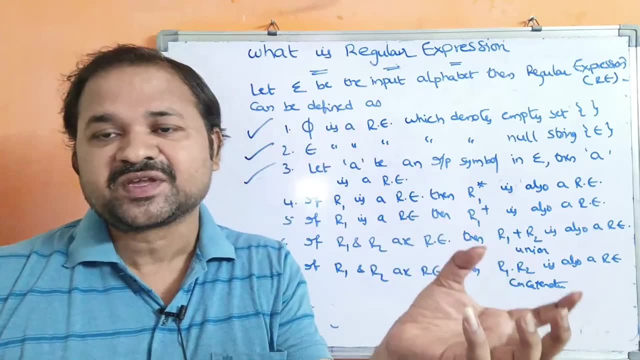 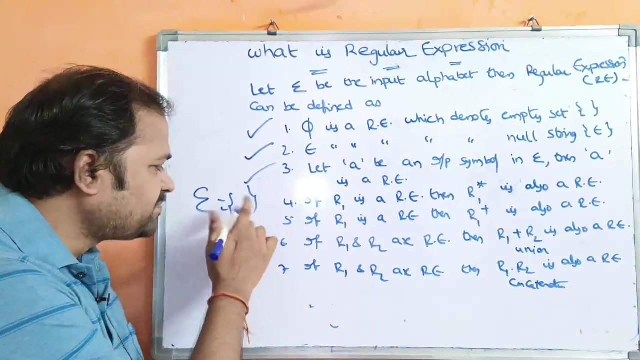 symbol in alphabet sigma, then a is nothing but a regular expression. So if we have an input symbol, a let sigma is equal to a, Then we can call this a as regular Let sigma contains x- input alphabet. x- input alphabet sigma contains a symbol called x. 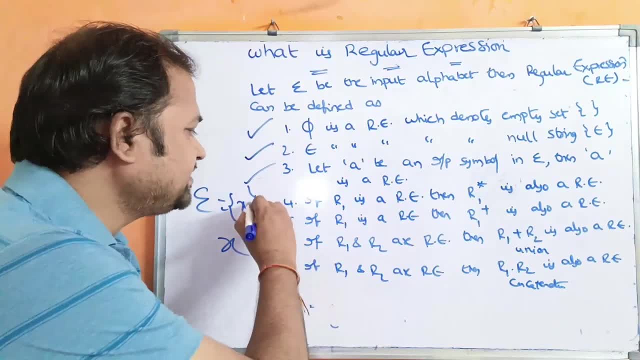 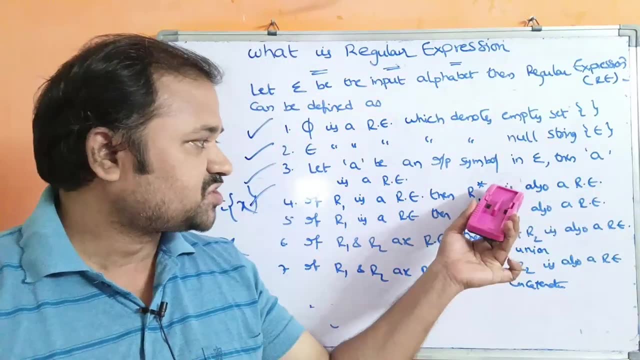 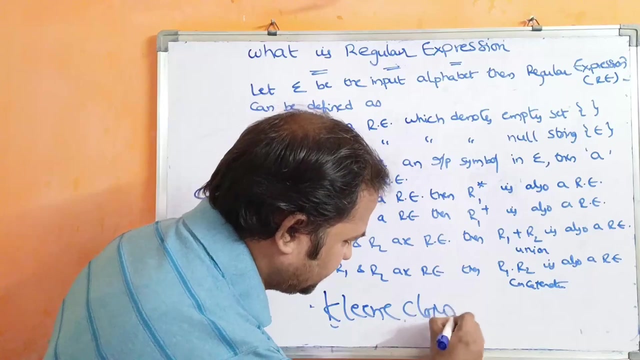 Then we can call x as a regular expression. Let us see the next rule: If r1 is a regular expression, then r1 star is also a regular expression Star. this star is called as clean closure, Clean closure, Clean closure. Let input alphabet contains a.